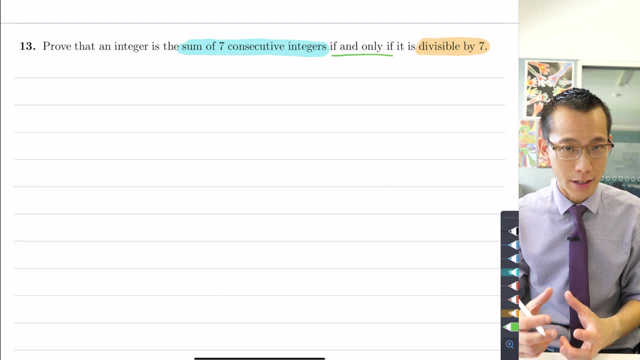 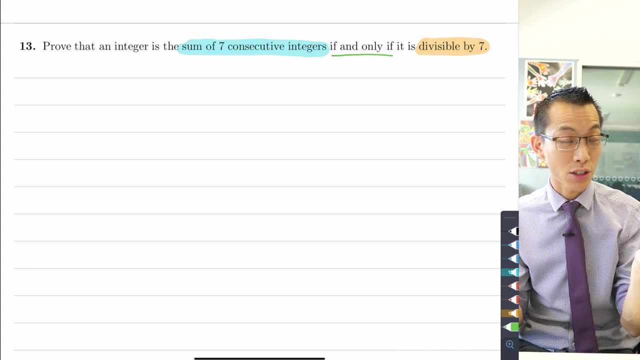 language that we use when two statements are equivalent, which is to say, one statement implies the sort of antecedent clause, implies the consequent clause, and also the same is true in reverse. The converse is also true. If you know the consequent clause, that also implies 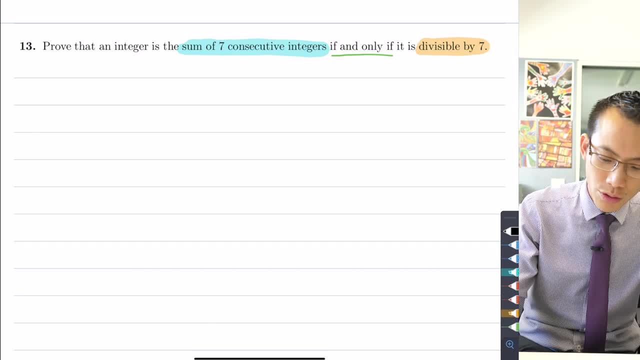 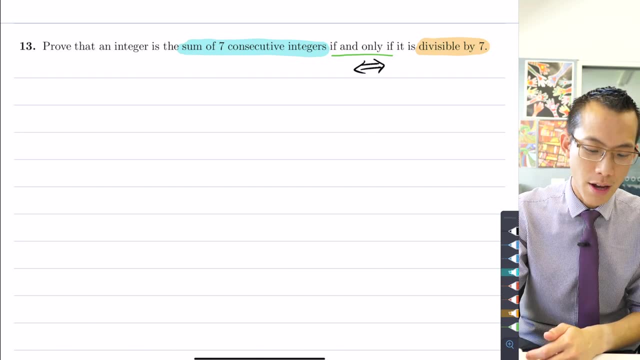 the antecedent clause. So I guess we would say that we could use this double-sided arrow here. right, That the implication is true and its converse is true. So not only is the sum of seven consecutive integers going to be divisible by seven, but you can also say any number divisible. 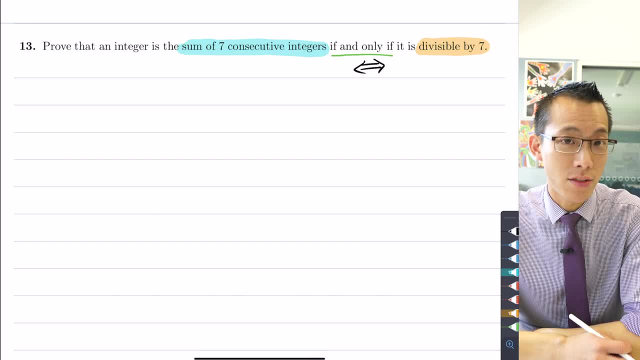 by seven can be written as the sum of seven consecutive integers, which is much less obvious. Now, in order to get at this, what I want you to recall is that actually, you've been dealing with equivalent statements. if, and only if, implication and converse are also true. You've 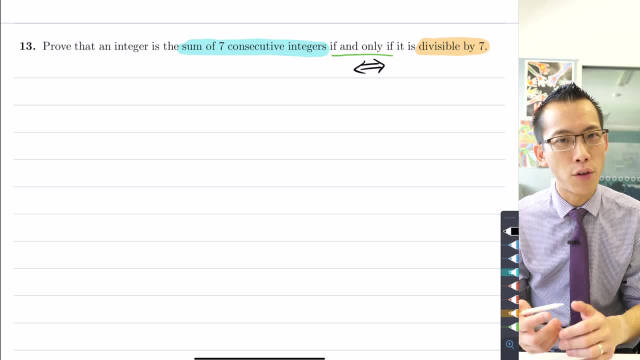 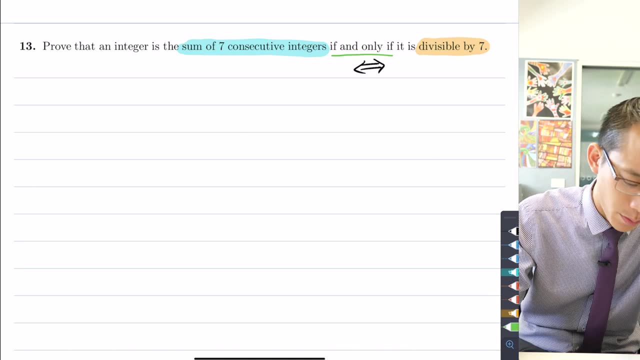 been dealing with them for years and years. We just never close them. in this formal language of proof, Let me give you an example to try and convince you of this. If I gave you, let's just go with green, because that's what we're trying to consider here. 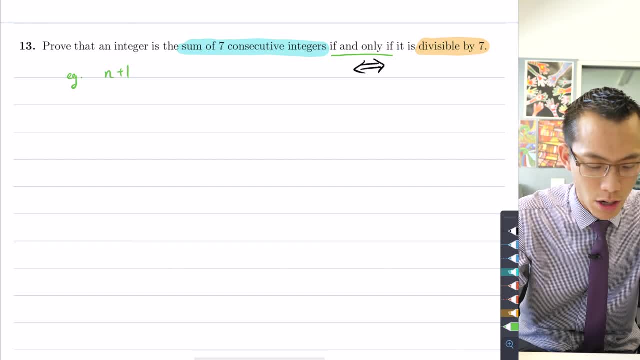 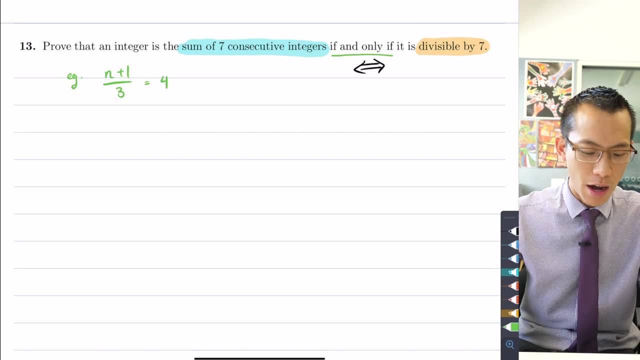 If I gave you some random algebraic statement like m plus one on three equals four, you're probably looking at this and thinking: well, this is not a hard thing to solve. I'm just going to try and make n the subject. So the most obvious first thing to do is multiply by three. 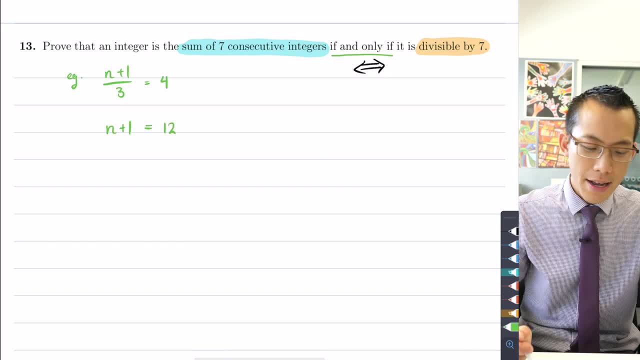 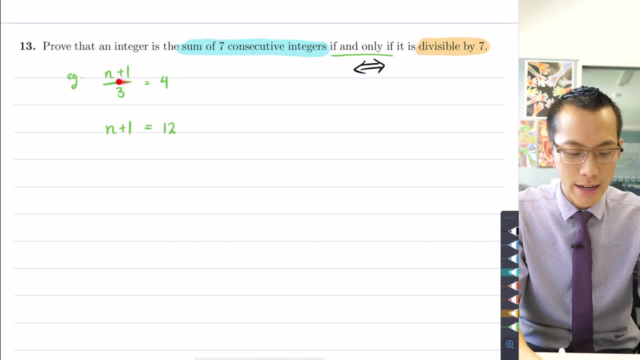 So if you did that, you would write this. Now here's what I want to get across to you, right? These are two different statements. m plus one on three equals four. It's a conditional statement, By the way. it isn't true for all values of n, It's only true for a certain value. 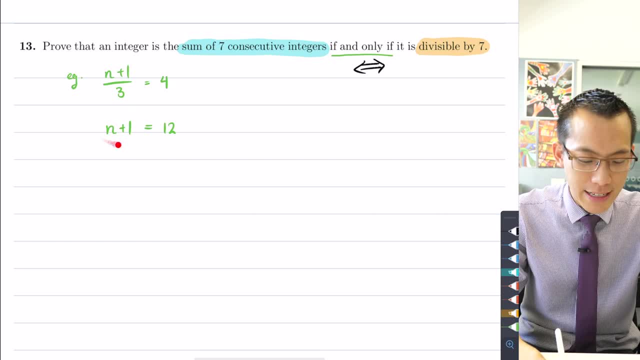 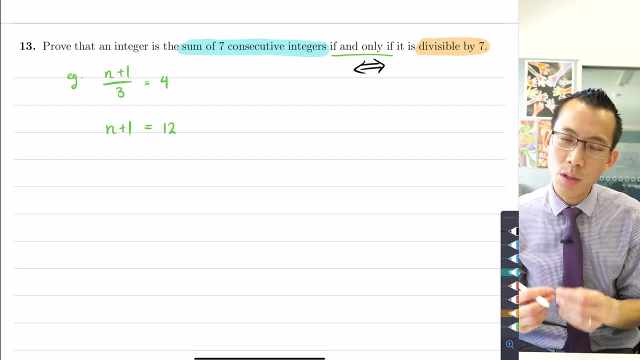 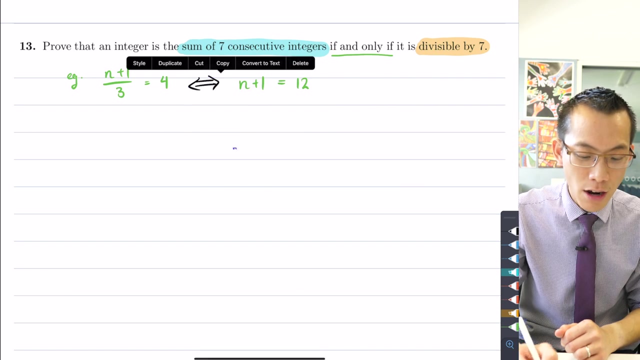 of n, namely 11.. But what you then write underneath this is its own statement, which is related to the previous one not just by arithmetic, It's also related by logic. Can you see that these two statements here are actually what we now call equivalent statements? If this is true, if this 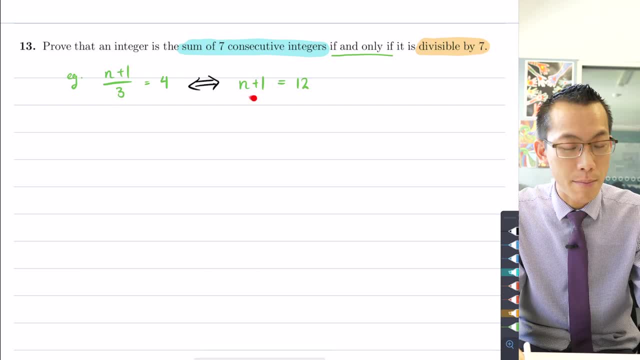 is true that m plus one on three equals four. it necessarily follows that m plus one equals 12.. But the converse is also true. There's no reason why you can't go in reverse: m plus one equals 12 also implies that m plus one on three equals four. I just have to divide both sides by three. 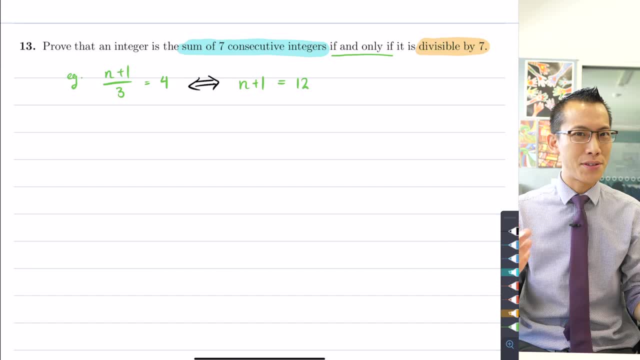 So what you can see here is that I don't know, in 99.99999% of all of the working in mathematical problems you've been doing, whenever you've written an equation and then written the next thing by doing some kind of operation to both sides, you've almost always been writing an if. 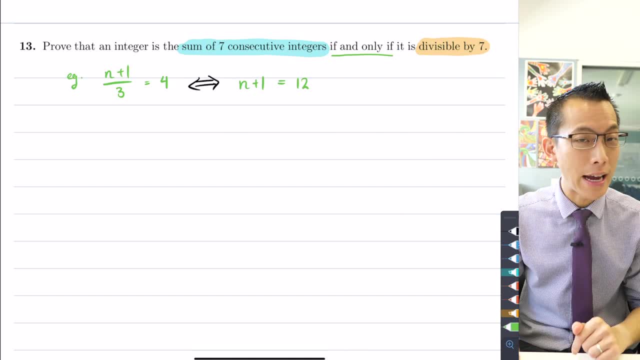 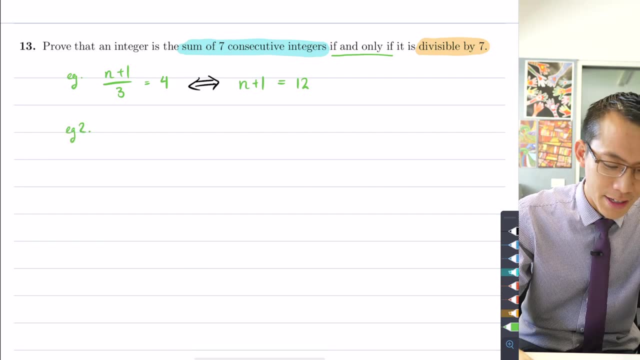 and only if statement. You've just never articulated it. Now, in a small number of cases, this isn't always true, And now we have the language to explain what's going on. For example, if I said to you, and just stay with me, even though this is like 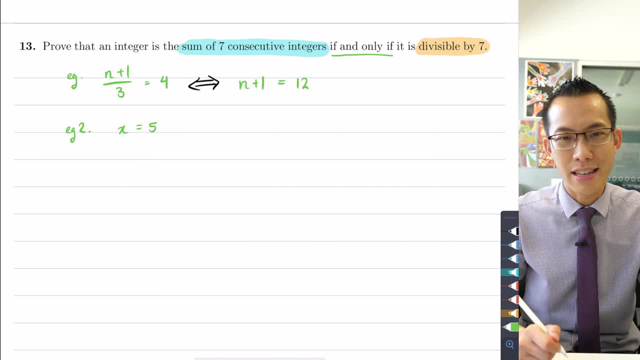 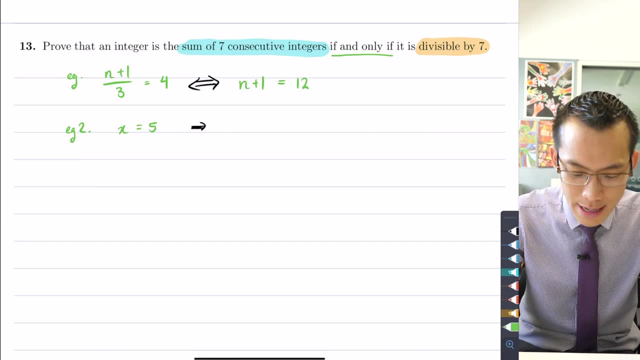 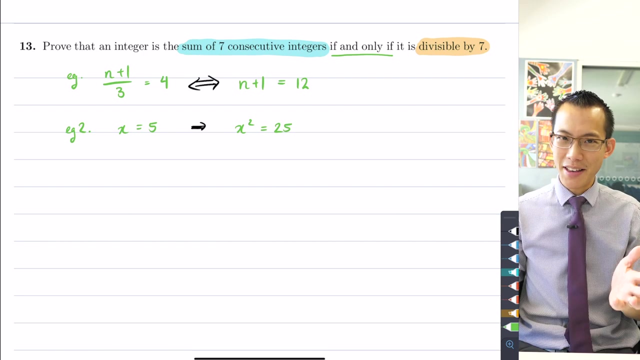 simple, just for the sake of illustration. suppose I said to you that x equals five, right? Does this imply? can I say that this statement will mean that x squared equals 25?? Just think about it for a minute And the answer is yes. of course it must If x equals five. 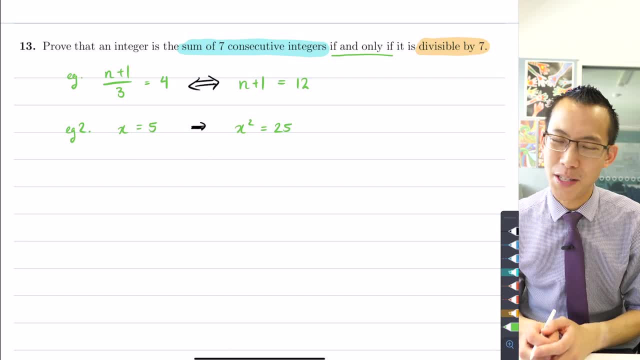 when you square it, there's nothing else you can possibly get. It has to be 25.. But this is not an if and only if statement. This is why we draw attention to it when we're first dealing with quadratic equations, that kind of thing. If I gave you instead. 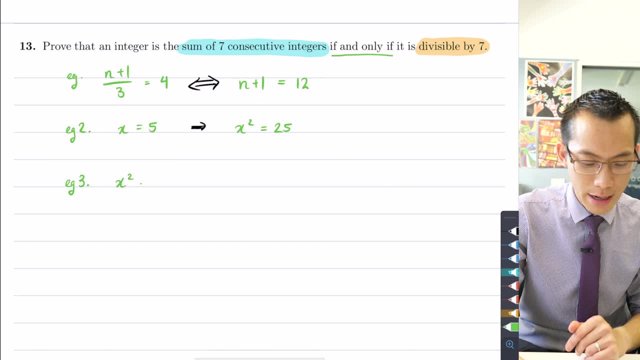 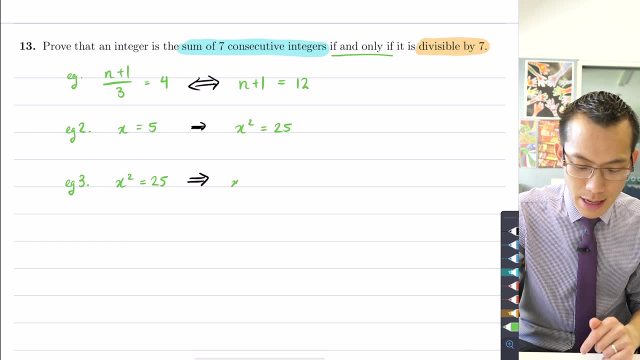 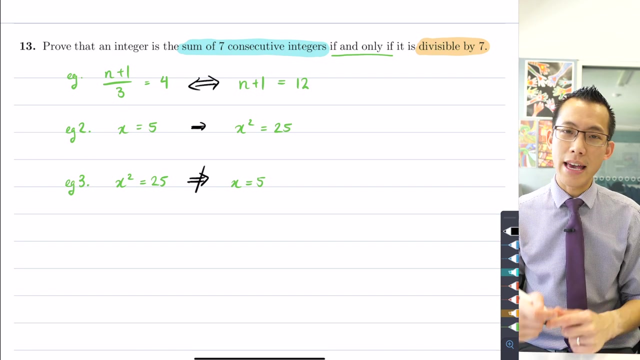 and this is a I'm going to treat this as a separate example. x squared equals 25, does that imply that x equals five? Is the converse of example two true? And the answer is no. it is not true, because x squared equals 25 implies there's another possibility. X can, of course, also equal. 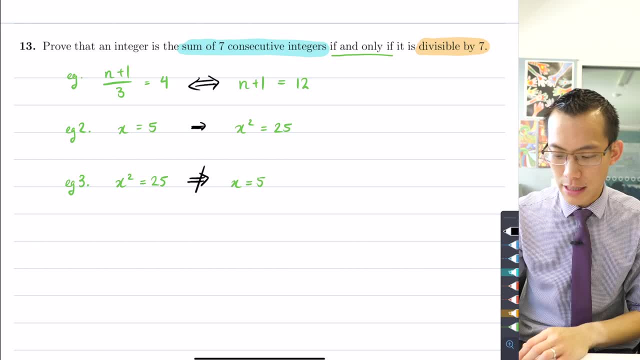 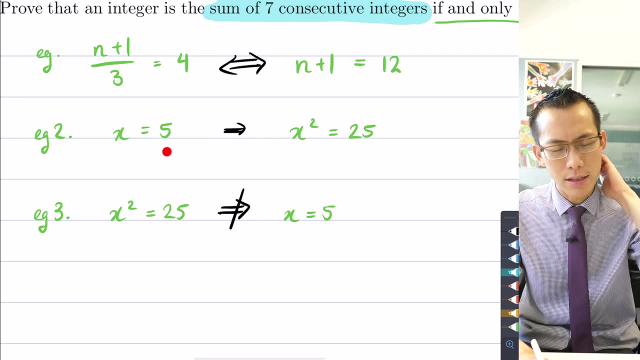 negative five. There's the negative case here, Right? So I guess what I'm trying to say here is: I'm trying to highlight that for some operations like, say, squaring and canceling as well is in a similar boat, right, You have to be very careful. 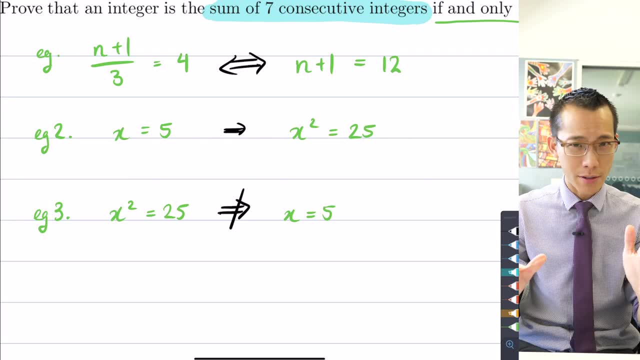 with the direction of your implication, And this is something that students famously get confused by when we're thinking about square roots, Why do we only take the positive value and not take both? And it has to do with the asymmetry of this logical statement. Okay, This is one of those. 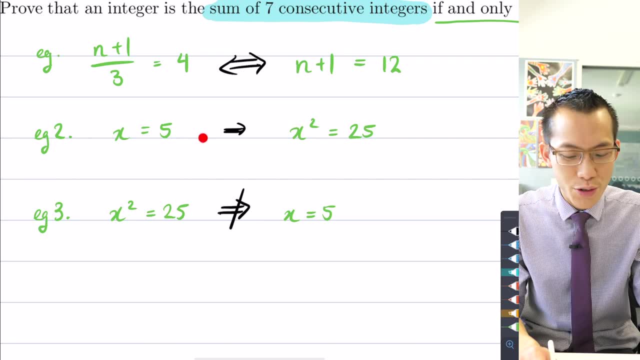 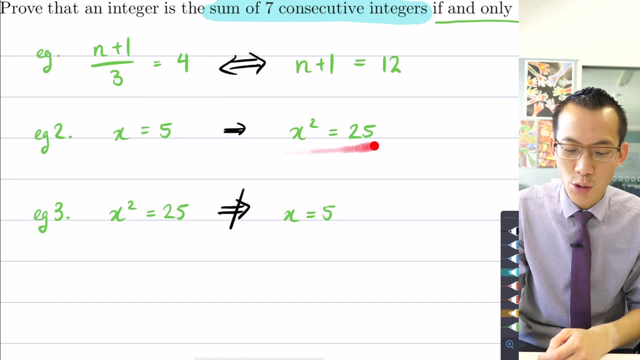 very few examples where one equation is not true if- and only if- it's related. you know sort of. I felt like I did the same thing to both sides. I just squared it right. This is one of the unusual cases. under most circumstances. 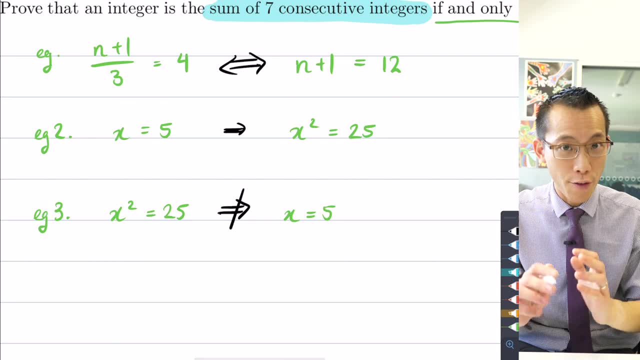 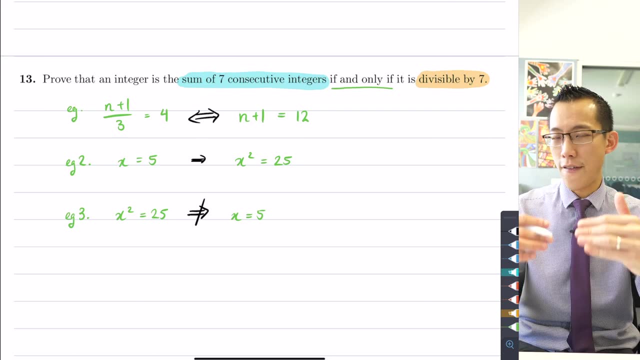 you know a lot of the work that we've been doing. I will fall under this case, and if only if. So what this means is: how do I prove an if and only if statement if I can do it through a series of fairly straightforward, if this is true algebraically? 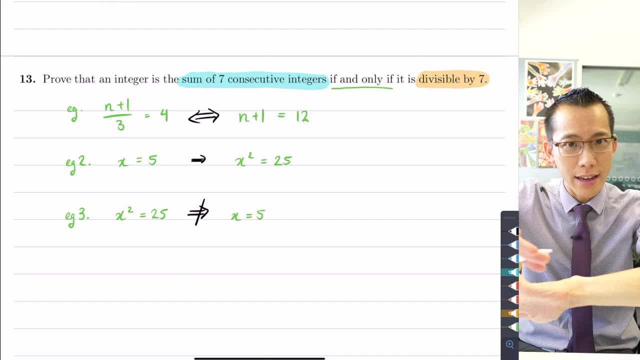 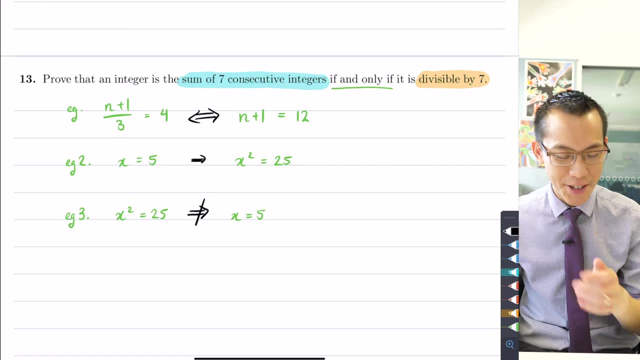 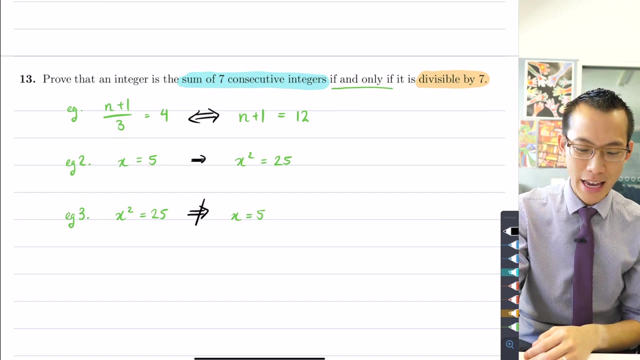 this equals this. then applying an operation- both sides, you know, preserves that, that truth. and then I've arrived at my if and only if. So now I've laid a foundation that basically writing equations that flow on one necessarily from the other is equivalent logically to saying a string. 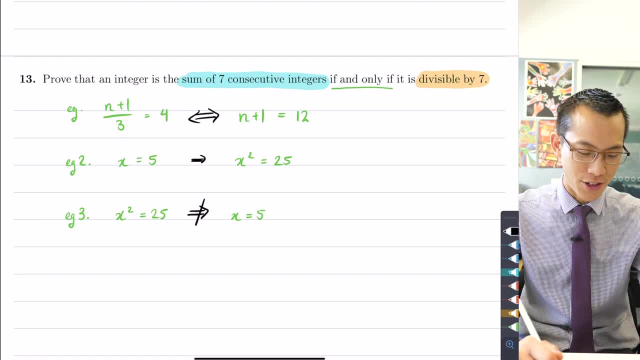 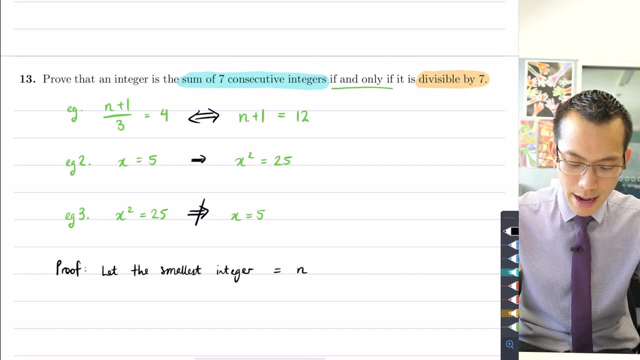 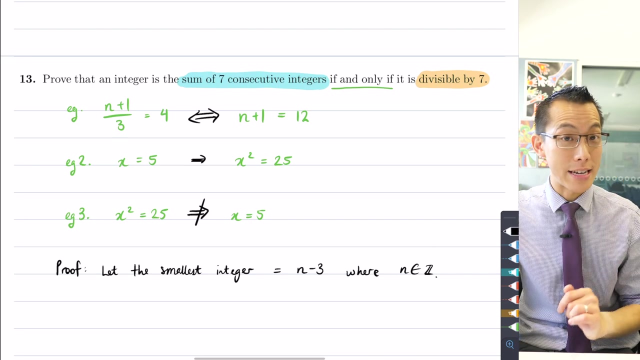 of if, and only if, statements. Now I'm ready to actually prove this question. Here's how I'm going to go about it. Proof: Let the smallest of the seven integers, let the smallest integer equal n minus 3n, Where, because I'm in integer land, I need to specify that n is an integer to make n minus 3. 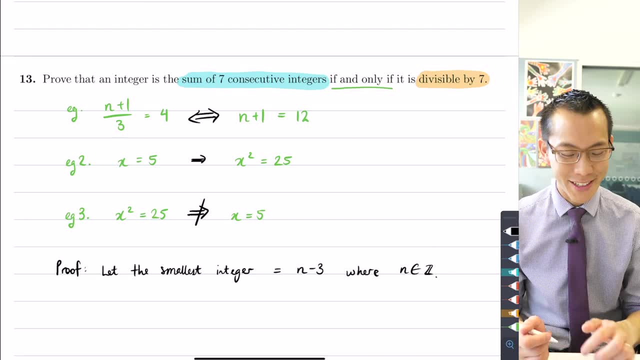 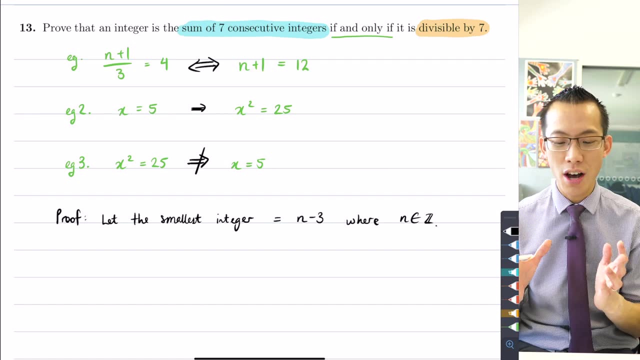 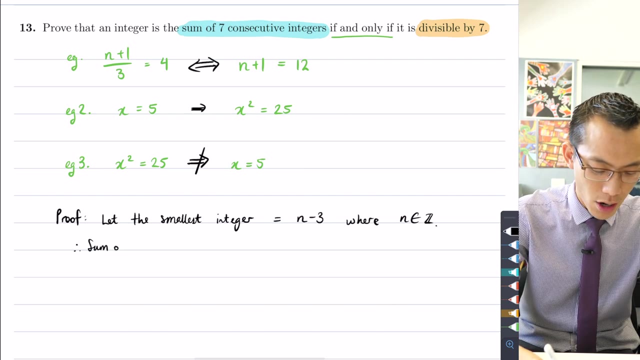 an integer. Now this might seem very random, but it's not going to be- in about 60 seconds. If the smallest integer is n minus 3, then it is not difficult to write the sum of the seven consecutive integers that start with n minus 3.. I can say, therefore, the sum of seven consecutive integers. 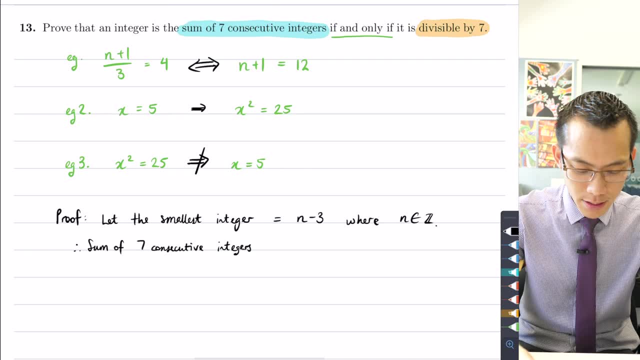 will equal what? And the answer is equals. I start with n minus 3, I'm going to put a bracket, set of brackets, around it to make it clear that that's one number, and then the next one along will be n minus 2.. I'm 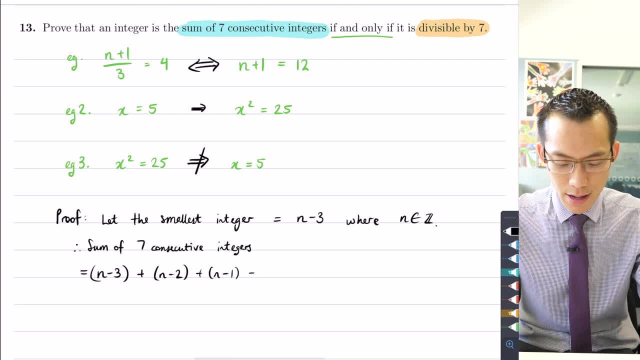 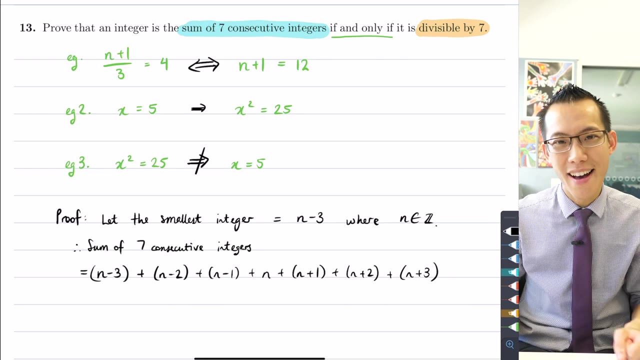 just incrementing by one, and then n minus 1, and then n. there's my fourth number, then I keep going in my adding one pattern. there's my fifth number, here comes the sixth one, and then here comes the seventh one. All right, so now you can see why. I hope I started with n minus three, because 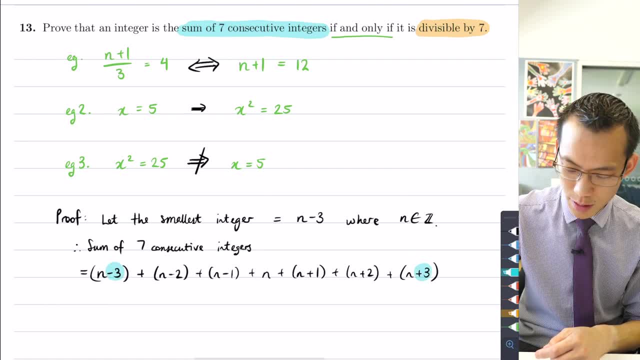 I want to get some cancelling happening. right, this minus 3 is going to cancel with this plus 3, this minus 2 is going to cancel with this plus 2, you get the idea. So what am I getting? It's just. 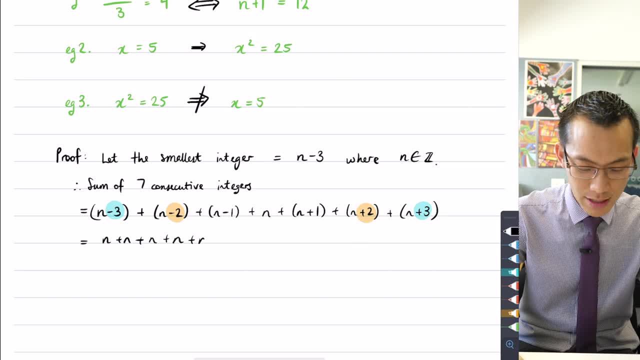 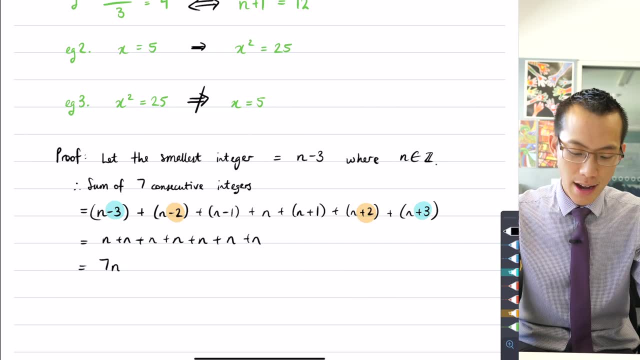 going to be n plus n plus n. I've got seven of these things because there's seven consecutive integers. so that's clearly equal to 7n. but I said n is an integer, so therefore 7n must be seven times an integer, that's a multiple of seven, ie 8n. Therefore, the sum of seven consecutive integers must be divisible by seven, because all multiples of seven by definition are, And because what I've done is I've gone through these equations, not doing anything dramatic, not doing any squaring or taking square roots.